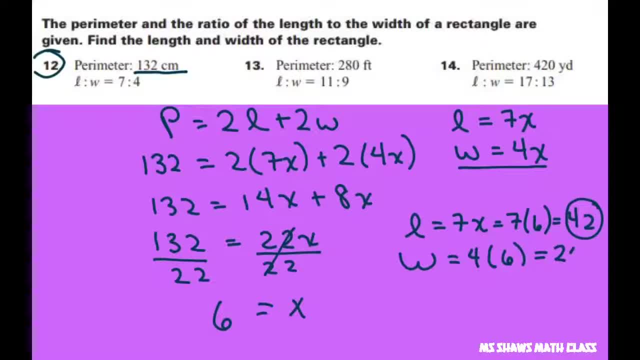 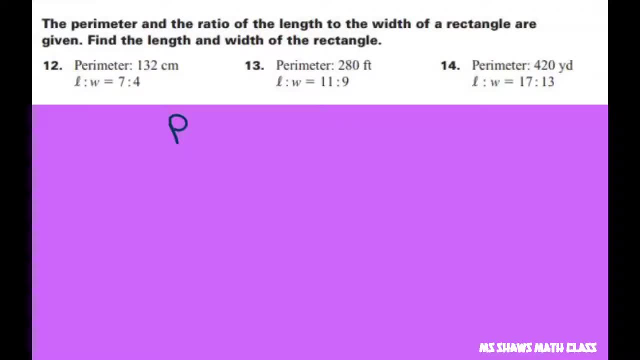 at this, which gives you 24.. And that's it on that one. Let's look at the next one. So next one, Write down your formula. Write down the length as 11X and the width as 9X, And the perimeter is 280 feet, So that's 2 times 11X plus 2 times 9X, And simplify. 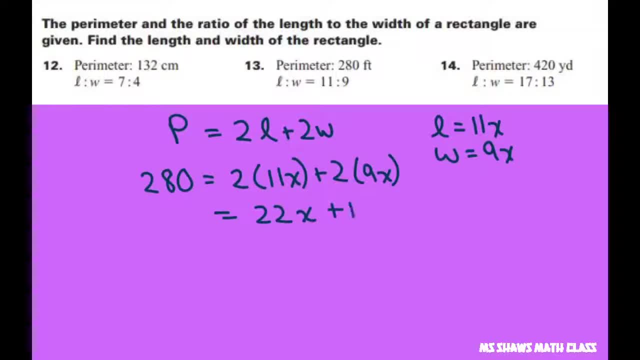 And you get 22X plus 18X equals 280 feet. 22 plus 18 is going to give you 40. Divide both sides by 40. And you get X equals 7.. Now the length is supposed to be in feet. 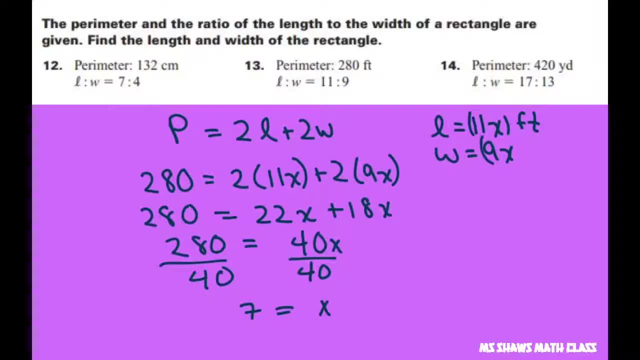 So this is really feet, This is feet. So just plug it in. The length is going to be 11X7, which is 77.. And just put your feet. I'll put it here: 77 feet And your width is not, which gives you 63.. 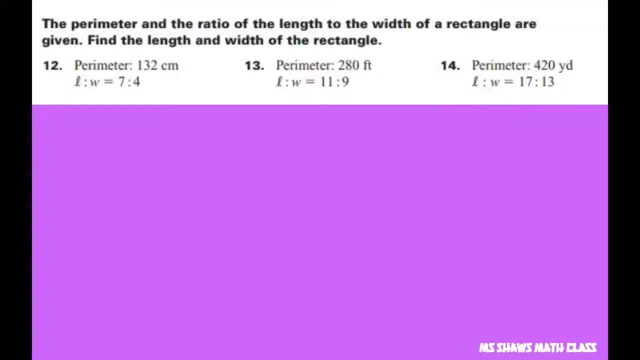 Feet. And for the last one, we're talking about yards. So we're going to let length equal 17X, And that should be in feet or yards. this time. Width is 13X And our perimeter is 420. equals 2 times L, which is 17X, plus 2 times width, which is 13X, And then we're. 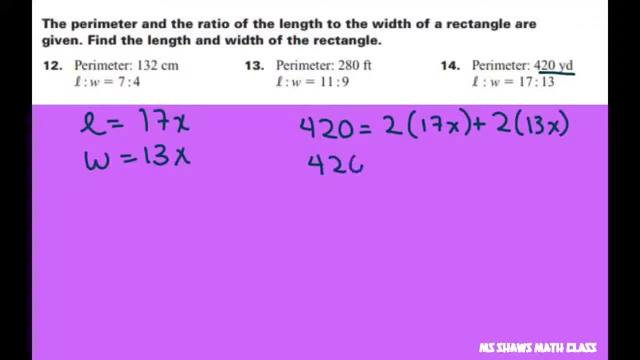 going to divide both sides by 16X. So 420 gives you 34X plus 26X, And 34 plus 26 equals 60. So you get 420 equals 60X. Divide both sides by 60. And you get X equals 7. Therefore.